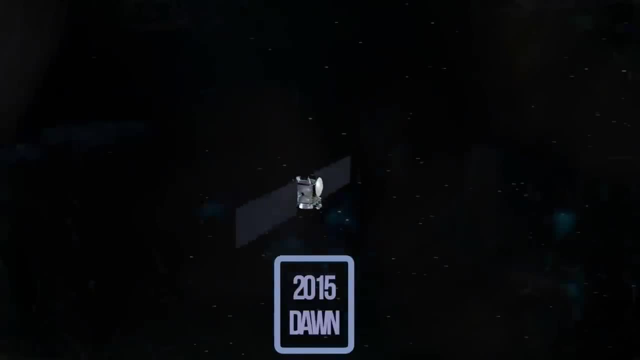 In 2015,. a spacecraft named Dawn orbited Ceres. That means it flew all the way around it In 2015,. a spacecraft named Dawn orbited Ceres. That means it flew all the way around it In 2015,. a spacecraft named Dawn orbited Ceres. That means it flew all the way around it In 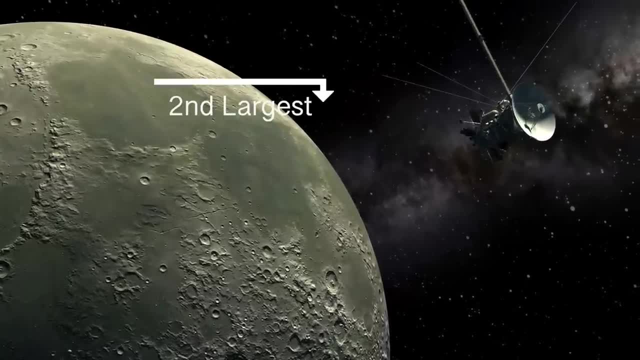 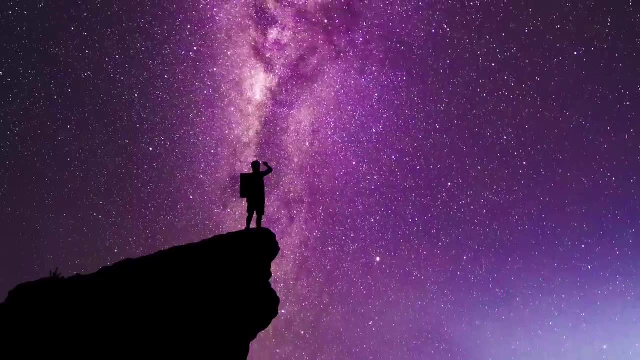 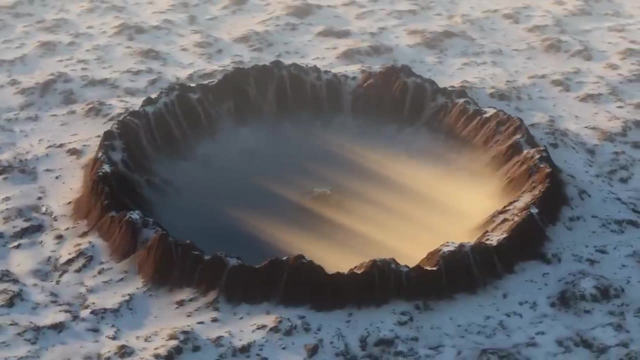 2011,. Dawn also orbited the second largest object in the asteroid belt. This asteroid called Vesta is the brightest asteroid in the sky. Every so often, it can even be seen from Earth without a telescope. Most asteroids contain craters or holes in their surface. Craters form when asteroids. 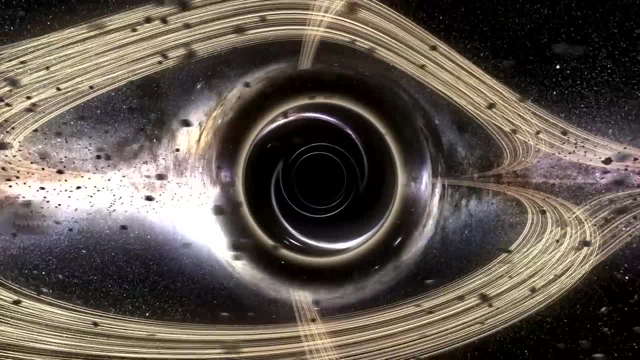 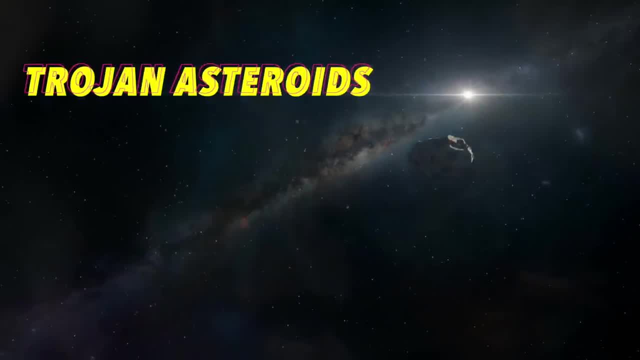 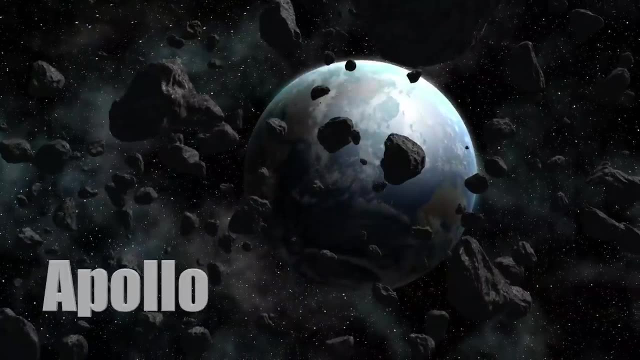 crash into other objects in space. Some asteroids have left the asteroid belt and spun into other orbits. These are called Trojan asteroids. Many move with the planet Jupiter as it moves around the Sun. Apollo asteroids are a group of asteroids near Earth's orbit. This group is made up. 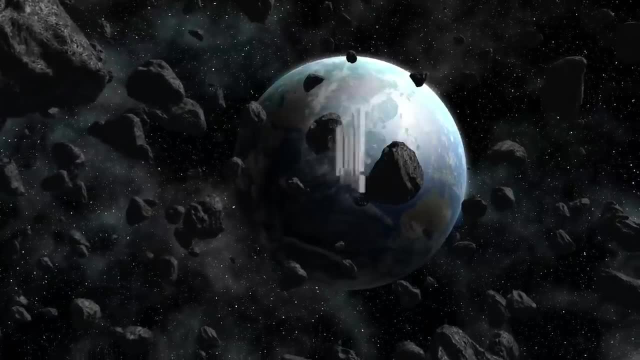 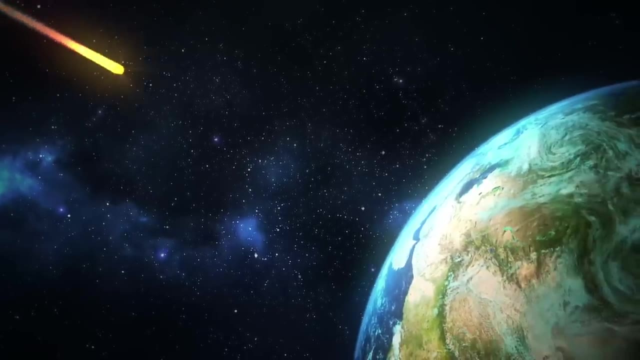 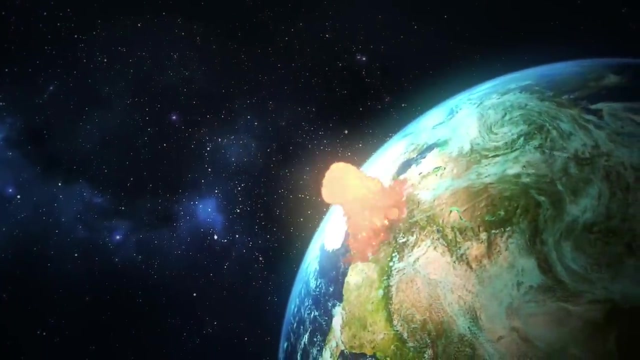 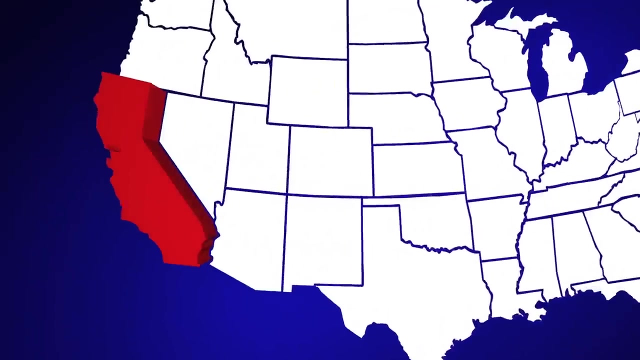 of over 10,000 asteroids. It is the largest group of objects near the Earth. Most of these asteroids burn up in our atmosphere, causing powerful blasts high up in the sky, But occasionally one of them falls to the earth. These are called Bolides or fireballs because they are so bright. Parts of Russia and California. 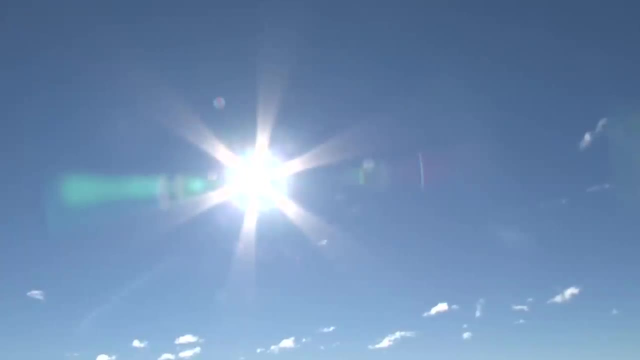 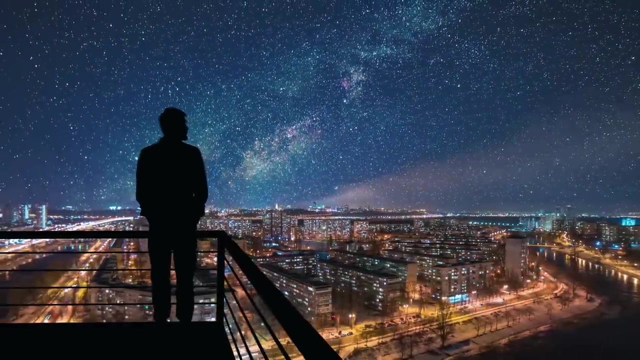 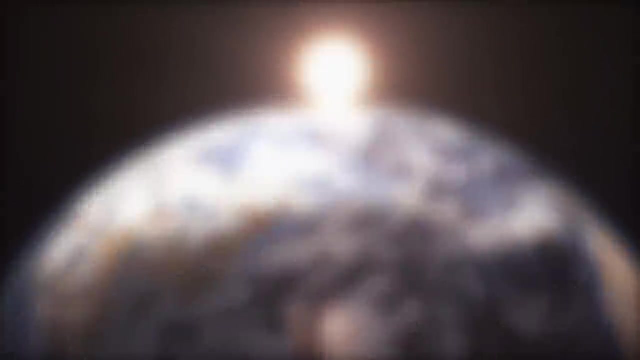 have been hit by Superbolides. These rare asteroids were 100 times brighter than a full moon when they fell. That would be an incredible sight to see. Comets are another kind of space rock. They are also bright. They look like shining lights. 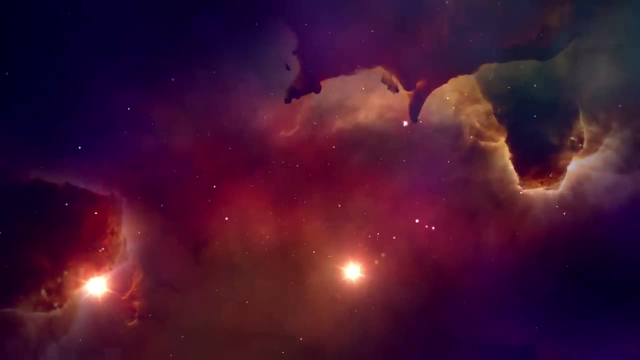 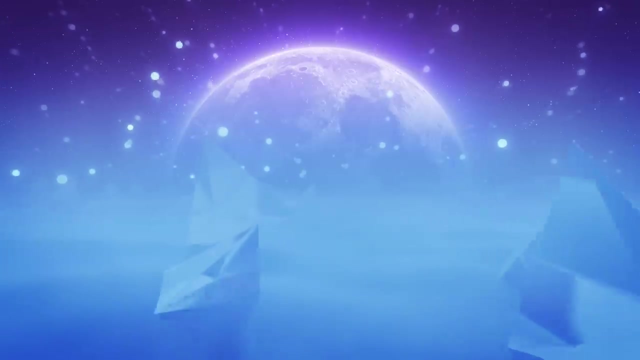 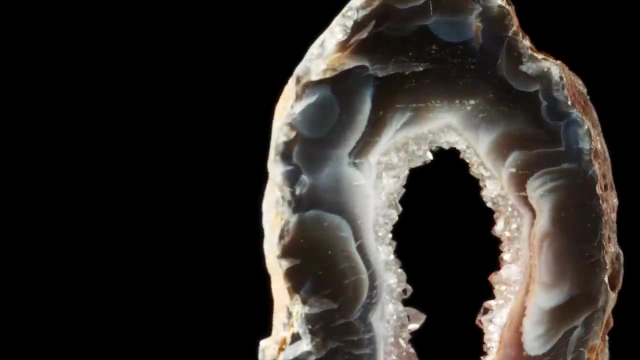 in the sky. A comet in the outer part of the solar system would be too small to be seen from Earth, even with a telescope. Comets have an icy middle, which is made up of water and gases that are frozen. They are mixed with bits of rock and metal too, and are covered by a layer of black dust. That's why they got their nickname: Dirty Snowball. When a comet gets close to the sun, the ice melts and changes into a gas Dust particles spread out around the center or nucleus of the comet. These dust particles create a cloud called a comma at the head of the comet. 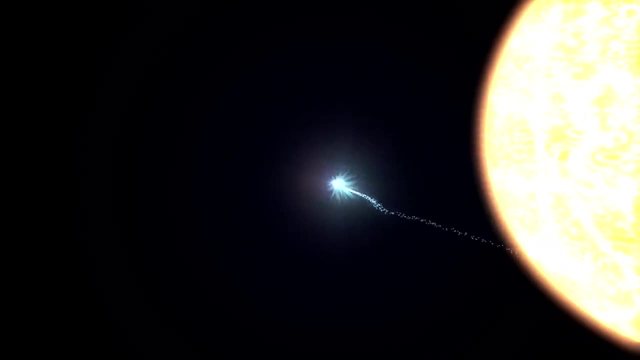 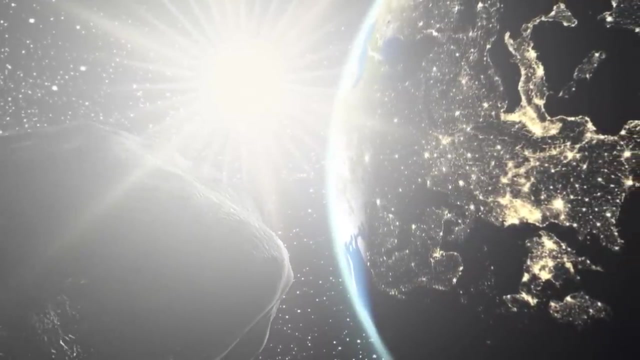 The sun then causes the comet to glow. A comet's tail can be millions of miles long. Some comets can be seen without a telescope as they pass the Earth near the sun. Comets come from either of two regions in the solar system. 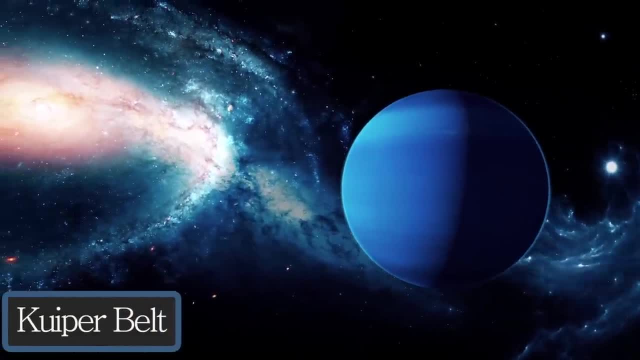 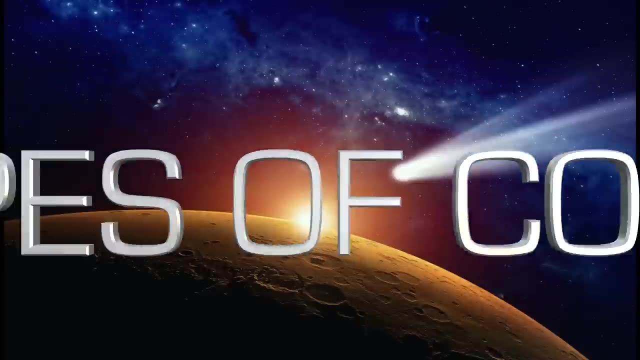 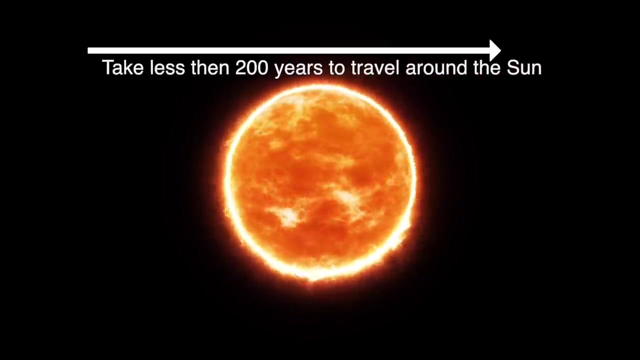 The Kuiper Belt, which is just beyond the orbit of Neptune, or the Oort Cloud, located beyond the outer boundary of the solar system. There are two types of comets: Short-period and long-period. Short-period comets take less than 200 years to travel around the sun. 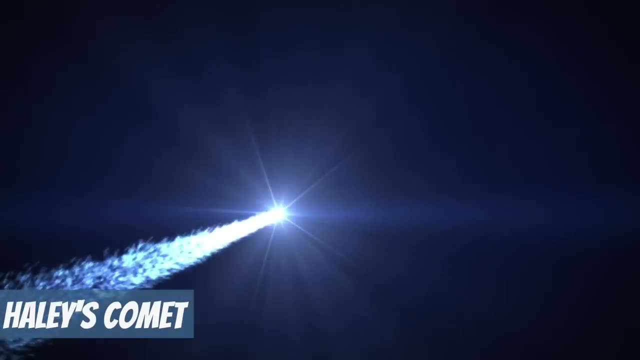 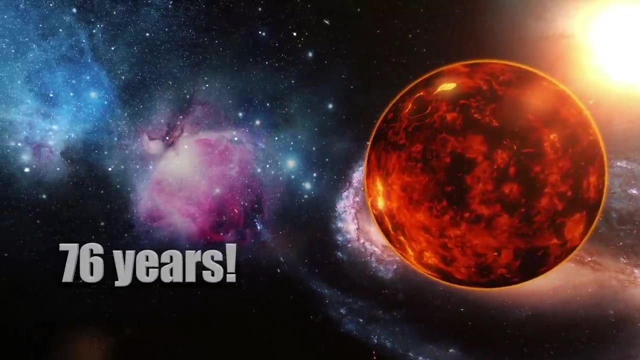 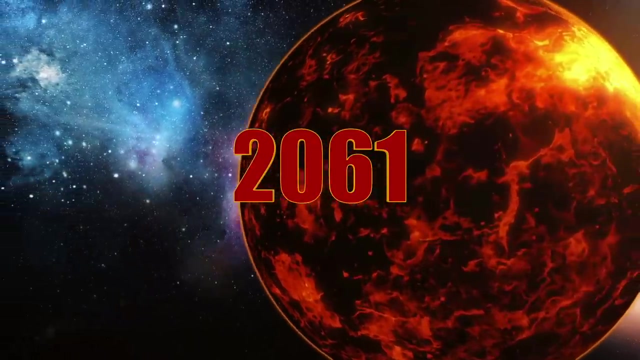 Two examples of short-period comets are Halley's Comet and Encke's Comet. Halley's Comet orbits the sun every 76 years. It was last year that the comet was born. It was last seen in 1986 and will again be visible around the year 2061.. 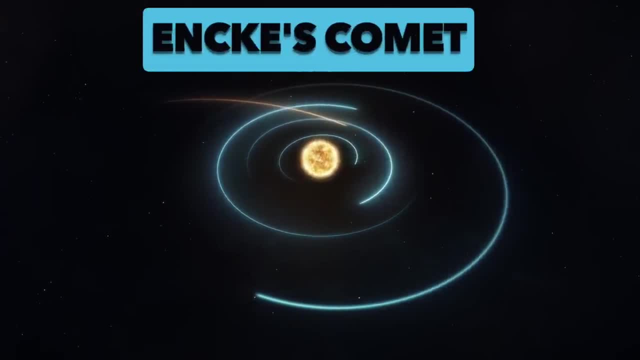 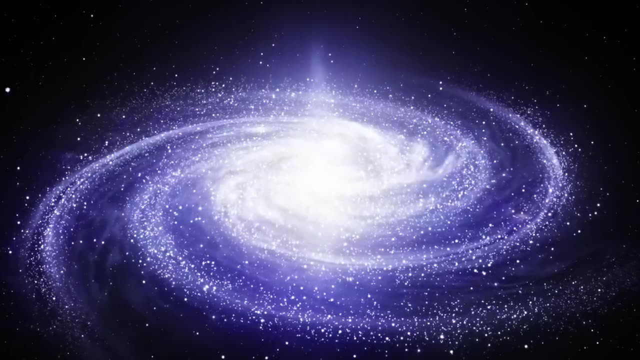 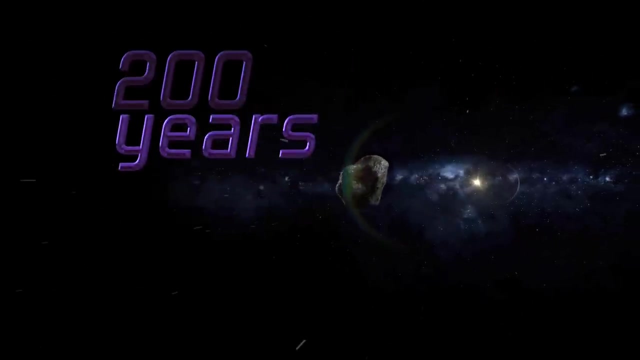 Encke's Comet has the shortest orbit of any known comet. It orbits the sun every 3.3 years. Both Halley's Comet and Encke's Comet originated from the Kuiper Belt. Long-period comets have orbits lasting more than 200 years. 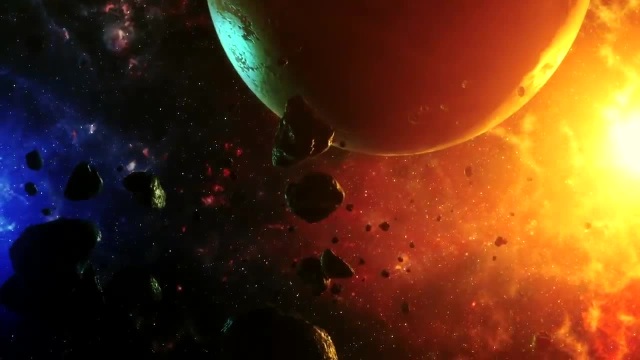 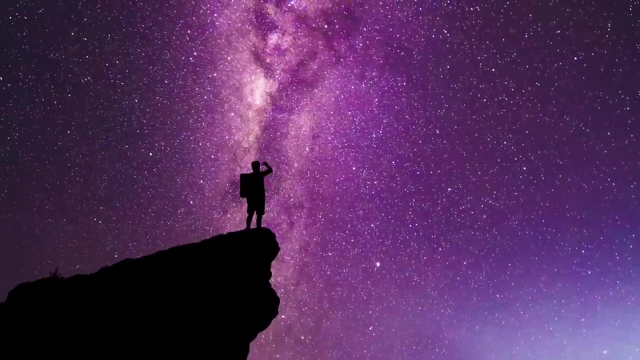 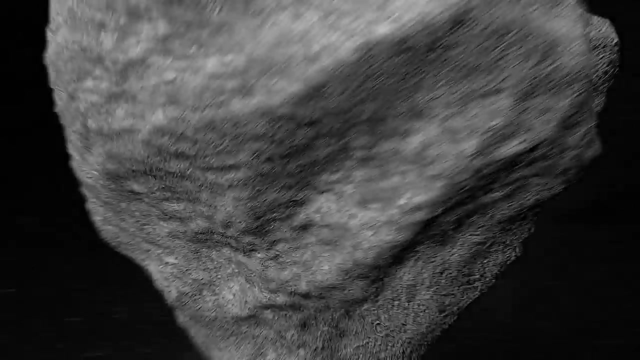 Some take more than 1,000 years. These originate from the Oort Cloud. Now let's discuss meteors. These rocks are sometimes called falling or shooting stars. They look like thin streaks of light in the night sky, But they are not actually stars. 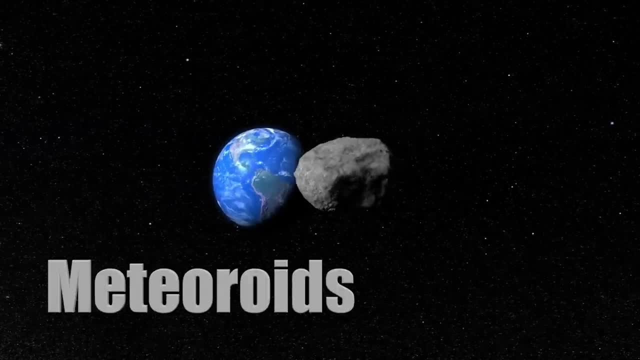 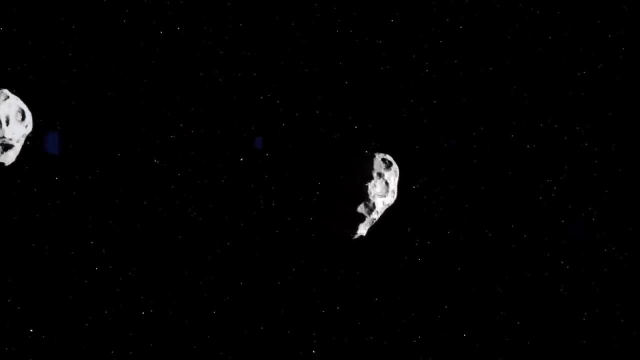 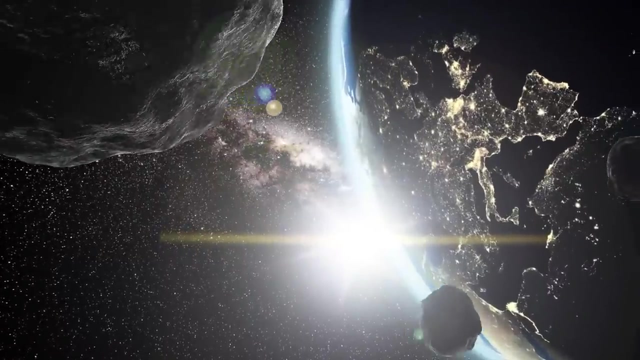 Meteors begin as meteoroids. Meteoroids are small pieces of rock or metal that break off a comet or an asteroid when they crash into each other. They can also form from the debris left behind a comet When these small pieces of rock are pulled into Earth's atmosphere. 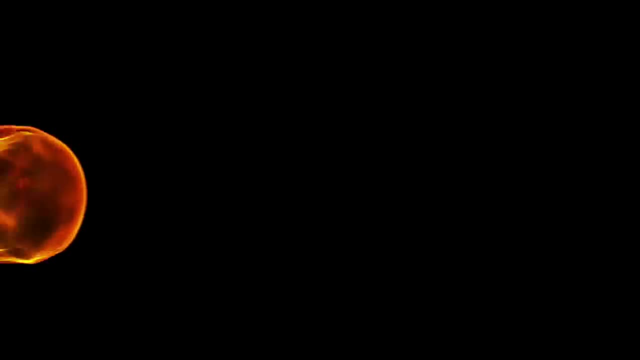 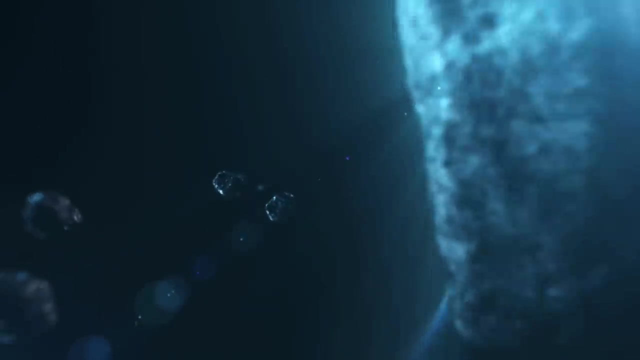 they are called meteors. The meteor heats up and burns, which makes them red-hot. If more than one of these meteors burn up, then you can see a meteor shower. A meteor shower looks like thousands of shooting stars falling from the sky. 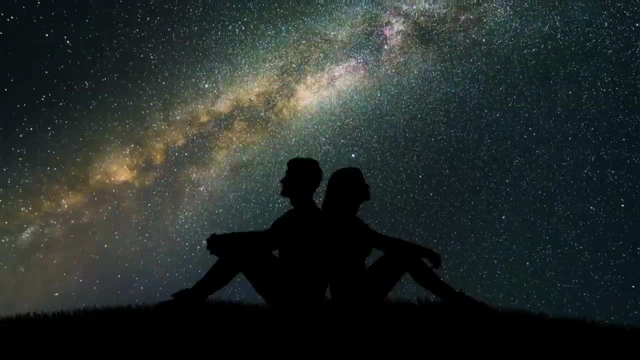 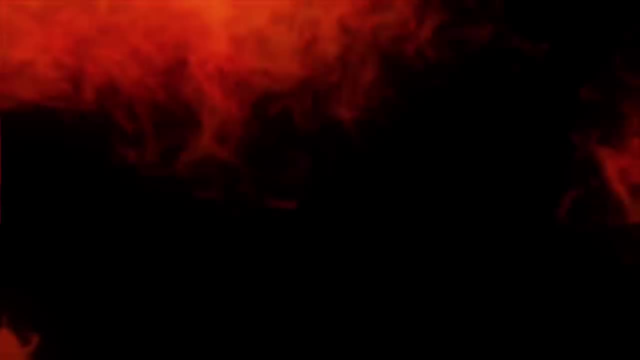 Meteor showers can be predicted throughout the year. If you get the opportunity to see one, don't miss it. They're really cool. Meteors only last for a few seconds before they burn up. A meteorite is a meteoroid that does not burn up in the Earth's atmosphere. 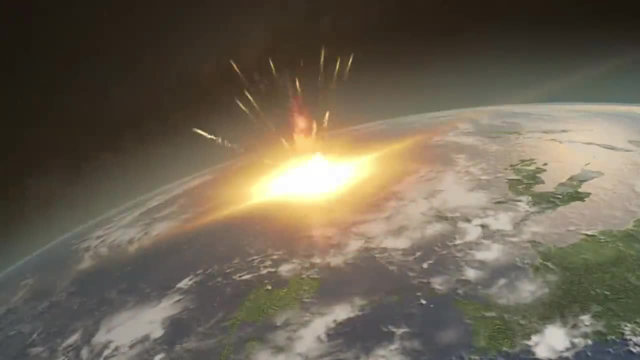 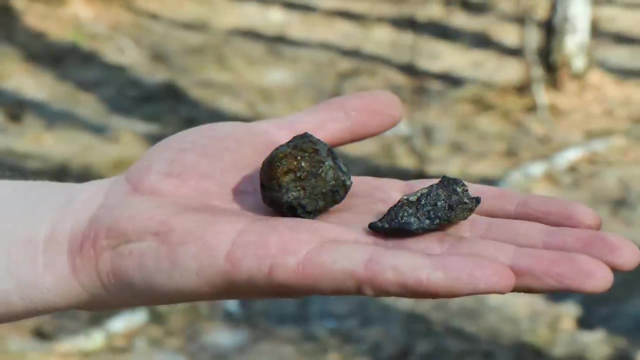 Instead, it falls to the Earth's surface. Millions of meteors enter the Earth's atmosphere every day. However, very few of them reach the Earth's surface as a meteorite. It's only about 500 a year, and most of those land on Earth. 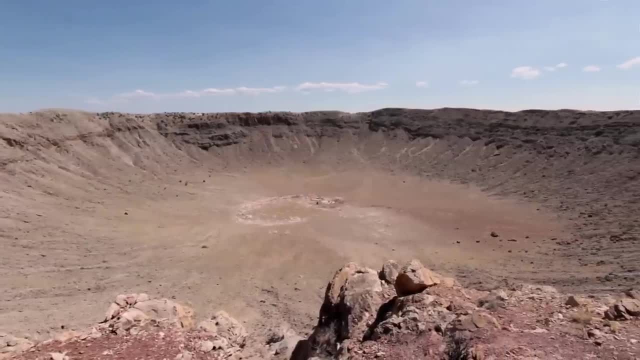 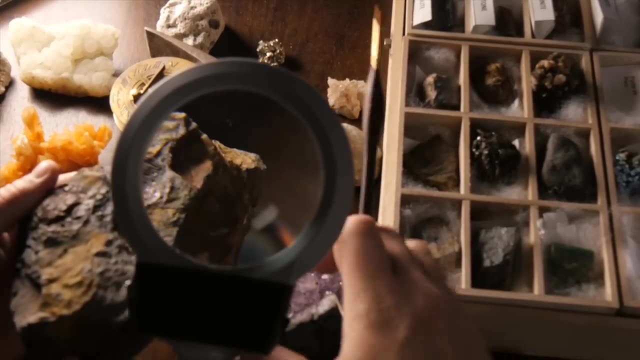 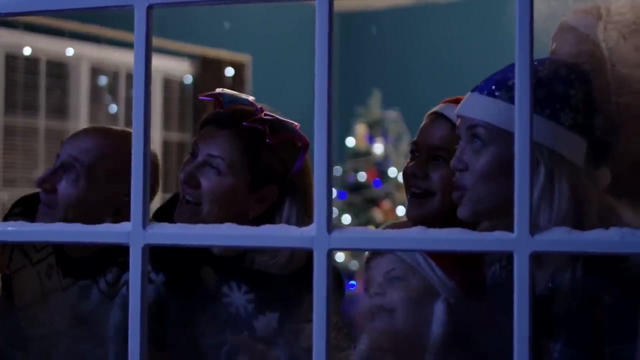 Although some have been found in deserts or in cold places like Antarctica, where the climate preserves them. over the years, scientists have collected more than 10,000 meteorites to study. The next time you look up at the sky, you just might get to see a meteor. 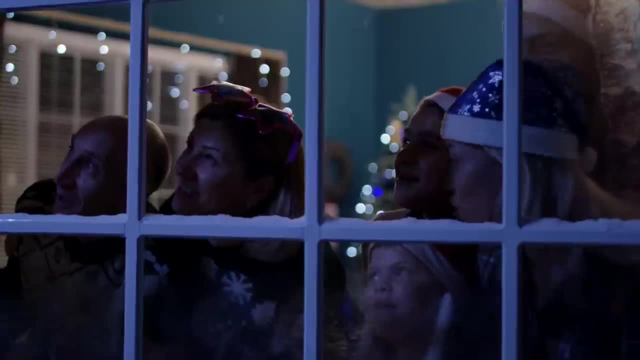 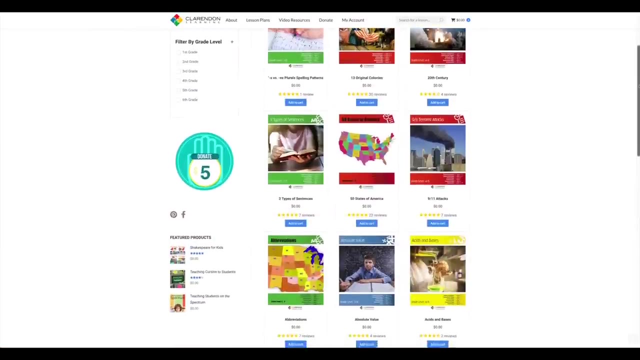 comet or an asteroid: Three pretty incredible rocks in our solar system. Thanks for following Clarendon Learning. Be sure to subscribe For more free resources. check us out at clarendonlearningorg. 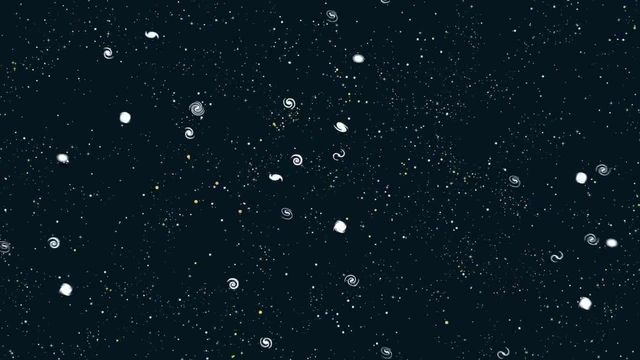 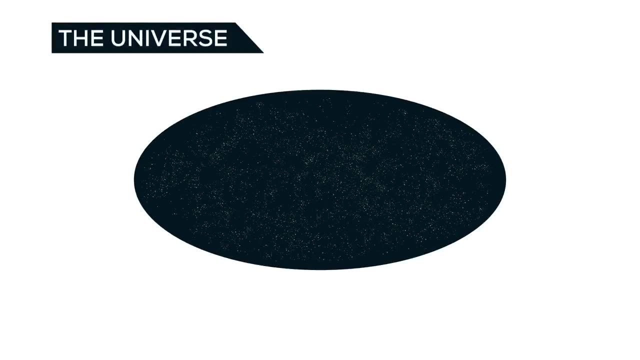 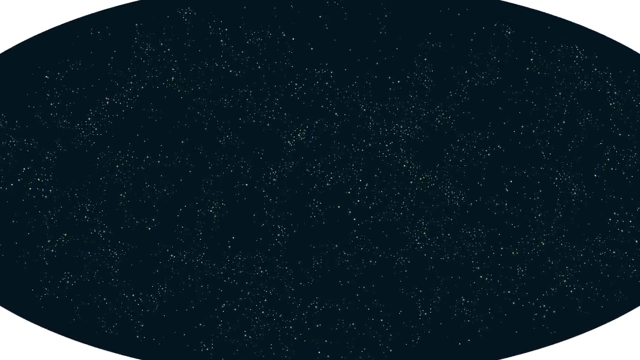 One day the universe will die, But why and how? And will the universe be dead forever? And how do we know that? First of all, the universe is expanding, And not only that, the rate of its expansion is accelerating. The reason: dark energy. Dark energy is a strange. 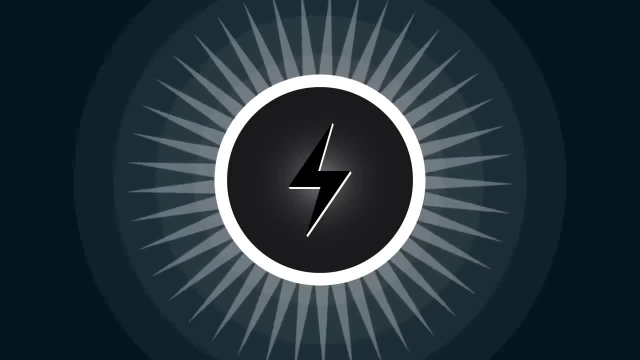 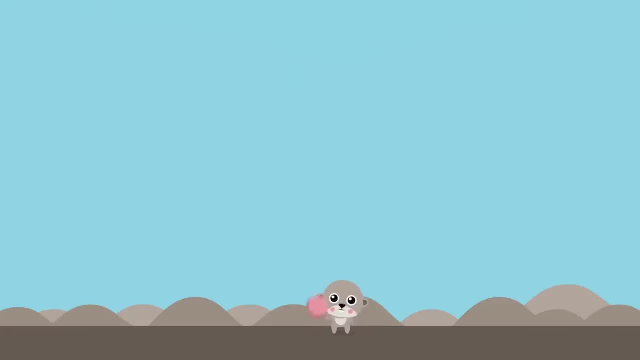 phenomenon that scientists believe permeates the universe. Until 1998, we thought that the universe must work a bit like a ball that you throw into the sky. The ball moves up, but at some point it has to come down again. But the expansion of the universe is actually 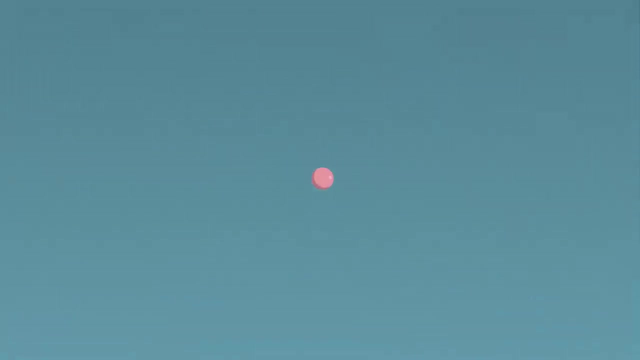 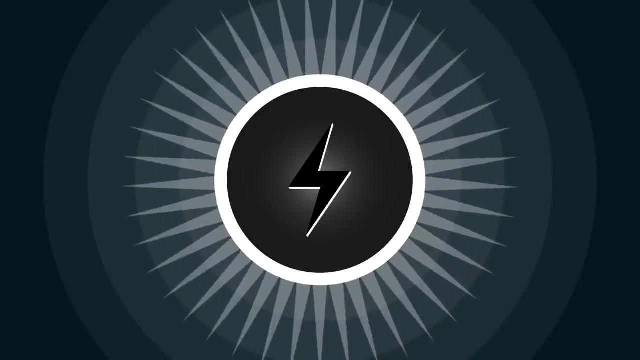 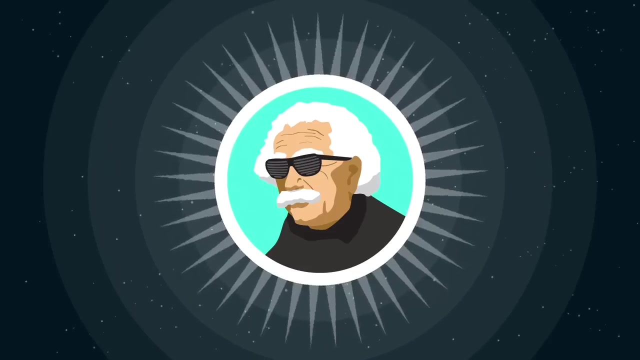 speeding up. That's like throwing a ball up and watching it fly away faster and faster and faster. Where is this acceleration coming from? Well, we don't know, But we call it dark energy. Einstein thought of it first and then decided it was stupid. 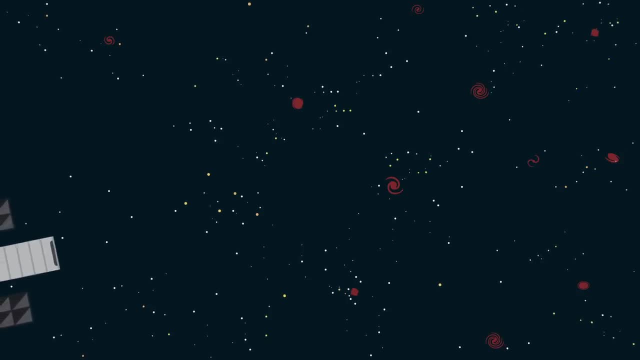 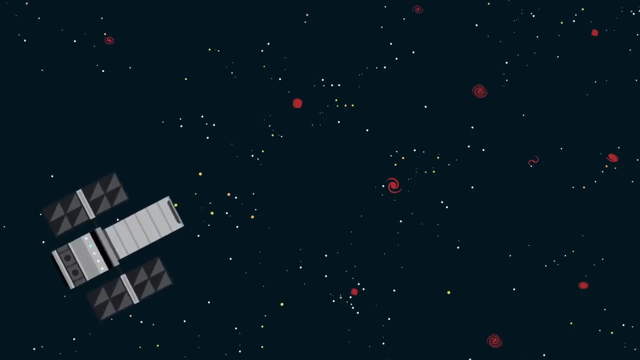 Now astrophysics. Astrophysicists have decided it is plausible. Trouble is, this is all very theoretical and we don't actually know what the properties of dark energy are. But there are various theories and they lead us to three scenarios for the end of the universe.